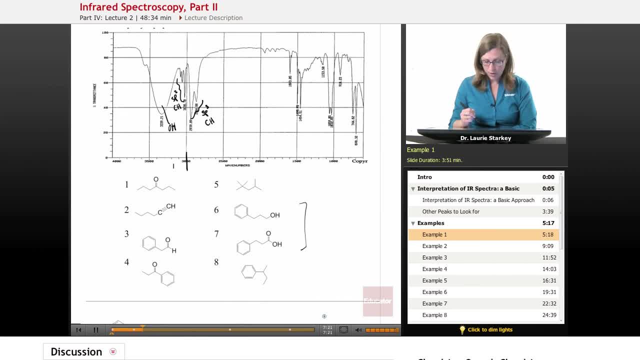 How would we distinguish between 6 and 7?? Well, there's two ways. One of them is: 7 must have a carbonyl, and we know we don't have a carbonyl. Right, we could just kind of make that note here: No carbonyl, Just as an FYI, I wouldn't really put that on my spectrum. Okay, but it can't be 7, so it must be 6.. It has the OH, It has the SP2CH, It has the SP3CH. Okay, now what else can we look for if we know it's 6 and we're thinking that it's 6.. Now let's go back to our structure. 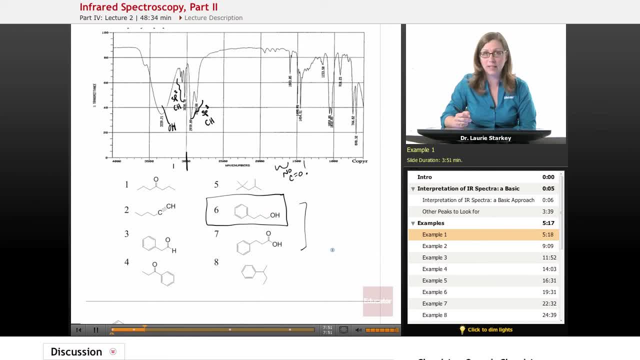 Let's go back and find some of those needles in the haystack that will more completely label this spectrum and give us further evidence, For example, because it has an aromatic ring. How would you describe that aromatic ring? It's a monosubstituted ring. So we in fact I see this aromatic ripple up here That's consistent with the monosubstituted 1,, 2,, 3,, 4.. And we also look to find, we should find two peaks around 700, 750.. And there they are. 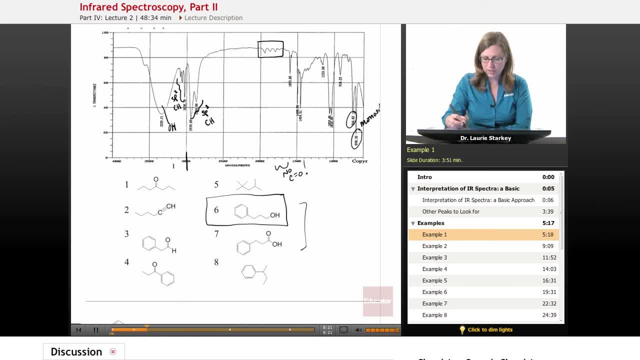 So this is monosubstituted aromatic. We call this the out-of-plane bending, So this gives us more evidence for that structure. Okay, is there anything else? Maybe we could look for that CO stretch, and maybe one of these is a CO I may. 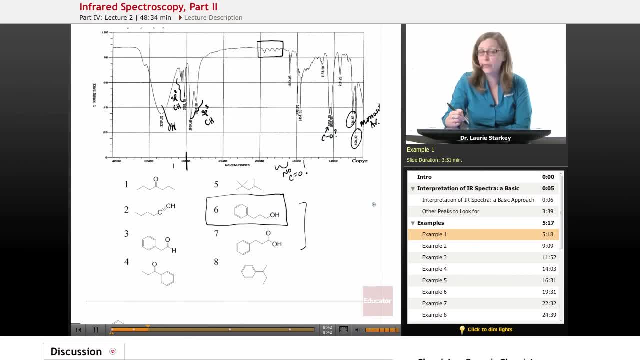 put a little question mark here. Right, there's two peaks here. I don't know for sure which is the CO. So you know that that's nice to attempt to label, but some things we're not going to be able to identify with certainty, Okay also. 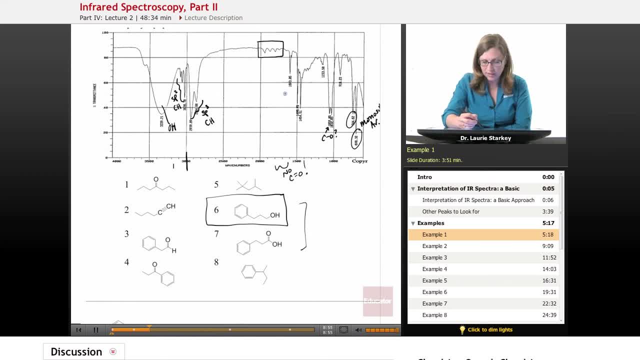 with the, with the benzene ring. maybe this peak around here at 1600 is the carbon-carbon double bond. You know, maybe we could put a little question mark there. I don't know, for sure that is. We would expect to find something. 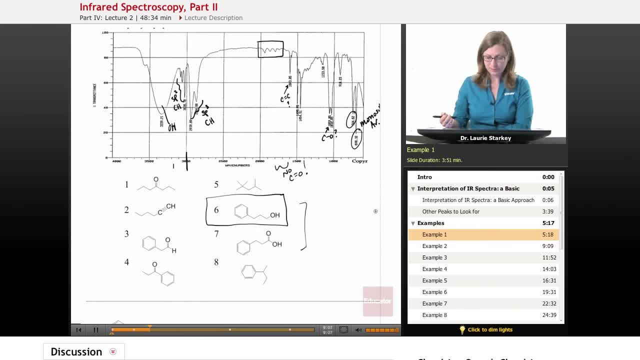 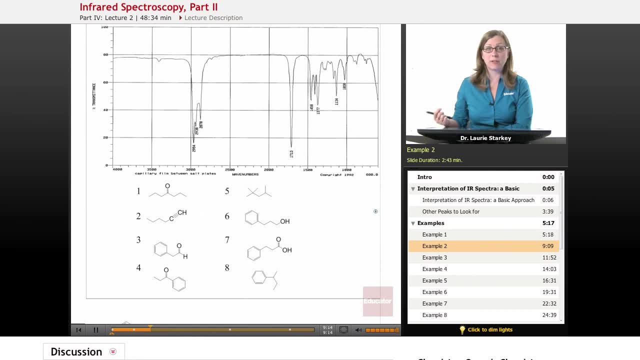 around that region. So that's probably a good guess. Okay, let's try another one. So we'll start by reading the spectrum from left to right. The first thing we should be looking for around 3300 is an alcohol. Do we have any OHs? Well, we have this tiny little blip, but that sure doesn't. 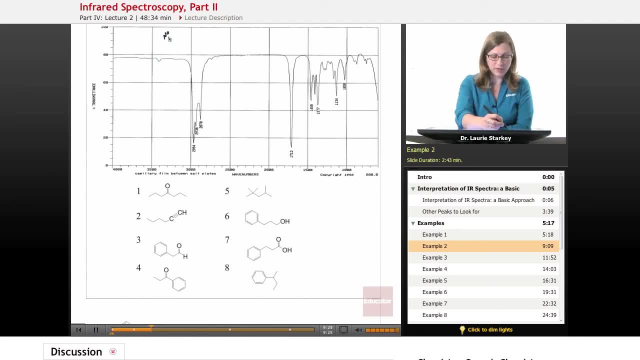 look like like anything significant. So we have no OH here. We continue to 3000.. Here's 3000.. We look just above anything, just above 3000. That's empty. So there's no sp2ch. We'll just put a little note up here on what we're seeing. How about just? 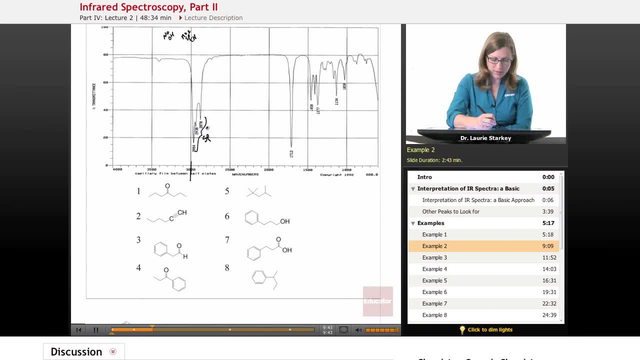 below 3000?? Yeah, here we have our first peak, significant peak, So we'll label those. We have sp3ch. We continue down reading left to right. at 2200.. Do we have any triple bonds? No triple bonds. And then we move down to 1700.. At 1700, what do we find We do have? 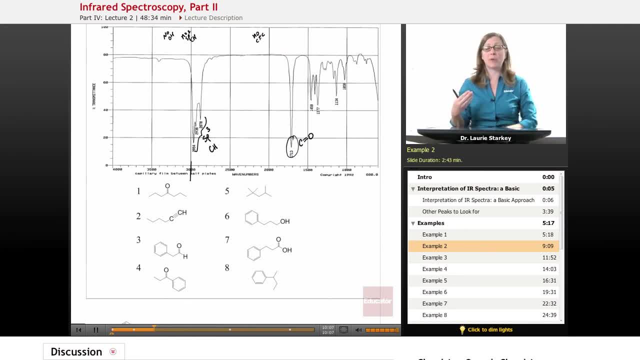 a carbonyl. Okay again, a systematic approach means we're going to be looking for our obvious peaks and we're not going to be missing them anytime they show up. So let's take a look at structures one through eight. What compound has a carbonyl and sp3ch and nothing else? Okay, so it can't be the 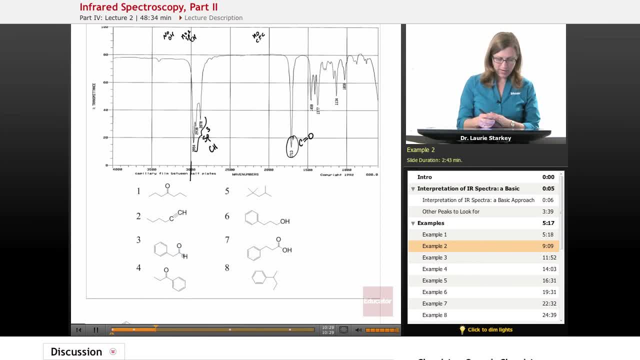 carboxylic acid because it had no OH, And we actually have three compounds with carbonyls Right, so we can cross these guys off as not being possible. These are our three contenders. How would we distinguish between them? These two are: 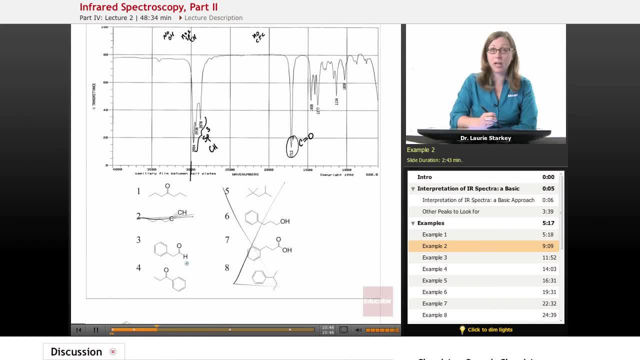 ketones. One and four are ketones and three is an aldehyde. And there's something else that distinguishes them. How about our ch's? We said that there's no sp2ch, but three has a benzene ring and four has a benzene. 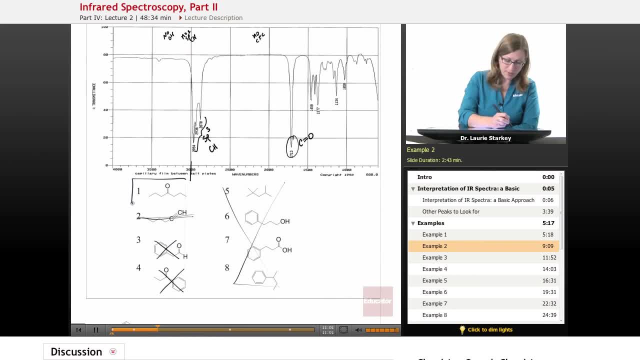 ring. So those cannot be our structure. So we actually have just one possibility here: This has to be this ketone, because all we have are sp3ch's and carbonyl. Okay, is there anything else I can look for to label? 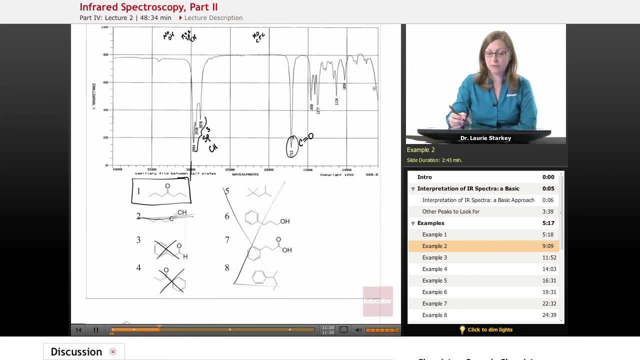 Re-. really, there's nothing else. So look at all those peaks in the fingerprint region that we're just leaving alone. Okay, sometimes that's going to be frustrating. You might find that frustrating, but the key to solving IR problems is knowing which peaks are significant, Being able to pick those out. 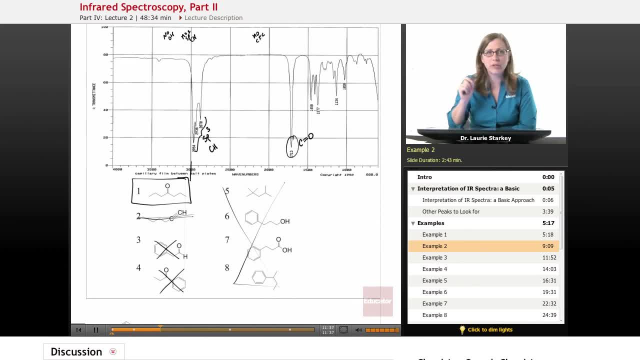 We have to resist the temptation to label every single squiggle and wiggle because they're just simply no, these are not significant peaks. It's simply your molecule bending and wobbling all around and that doesn't really tell us anything diagnostic. Okay, so just those two peaks are all we need to label and to positively identify its structure. 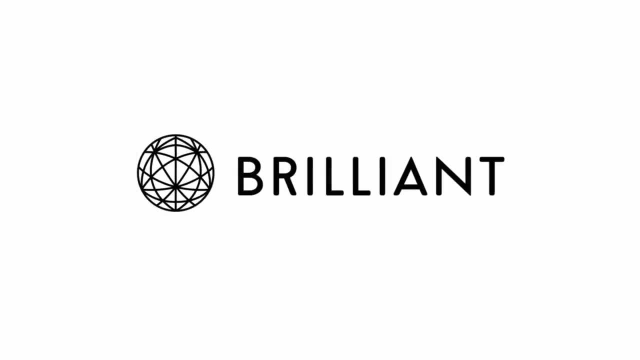 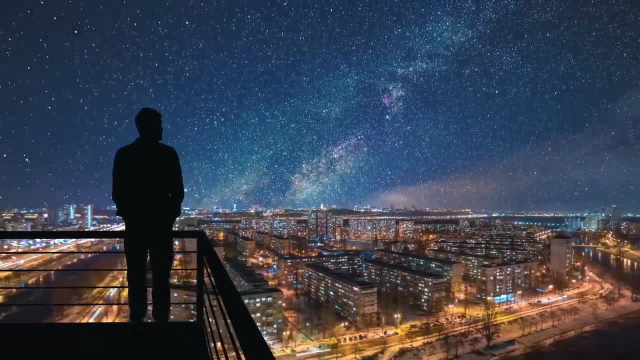 This video is sponsored by Brilliant. Stay tuned to the end for a special offer for Arvin Ash viewers. In physics, there is one ultimate goal, and that is to describe the world we are in. The hope is that one day we'll find some underlying theory that connects 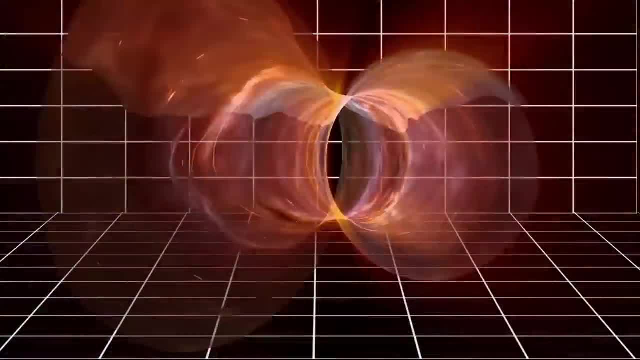 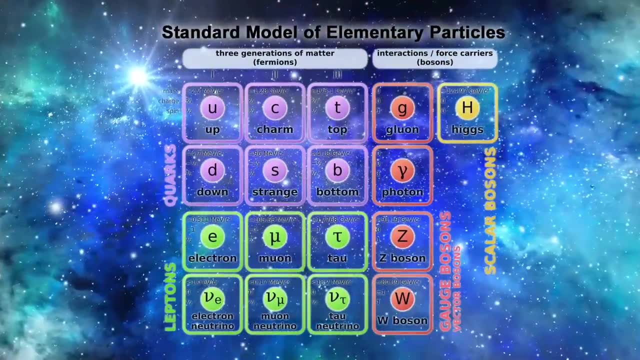 all the little pieces into a grand puzzle forming a theory of everything, The ultimate theory describing the world we find ourselves in. So far, the closest we have gotten to this is the standard model of particle physics. This is like the periodic table of elements. 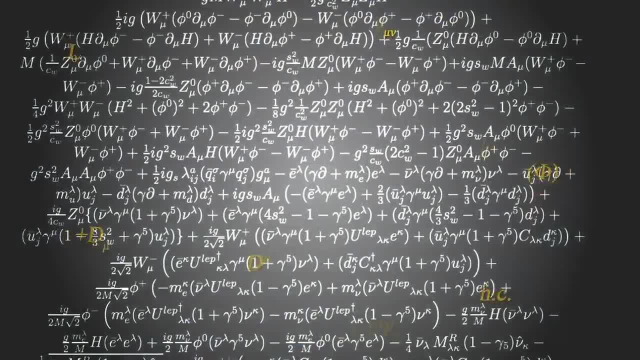 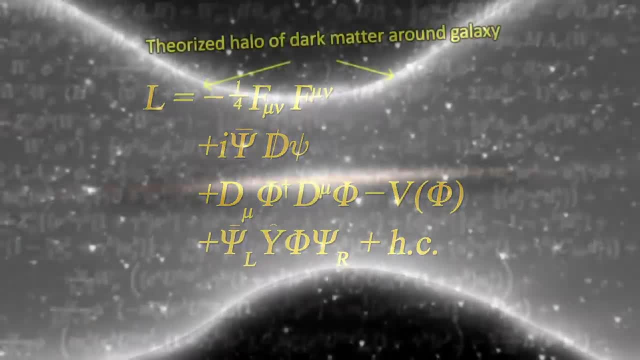 for fundamental particles, And the equations behind this theory are the most accurate we have ever had in physics. It's pretty good, but there are a lot of missing pieces, Things that the theory just doesn't account for, like dark matter, dark energy and a quantum theory of. 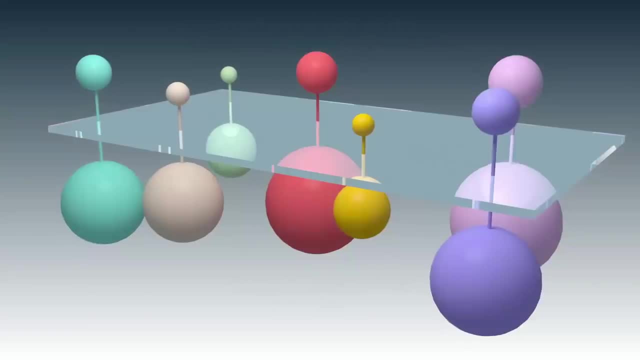 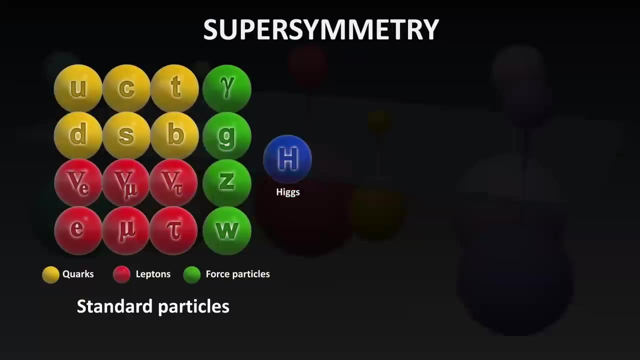 gravity as well as several other issues. But there is a theoretical idea that many people think could get us closer to a theory of everything and could fill several gaps in the standard model. This theory is called supersymmetry, which is the idea that matter particles and force-carrying.